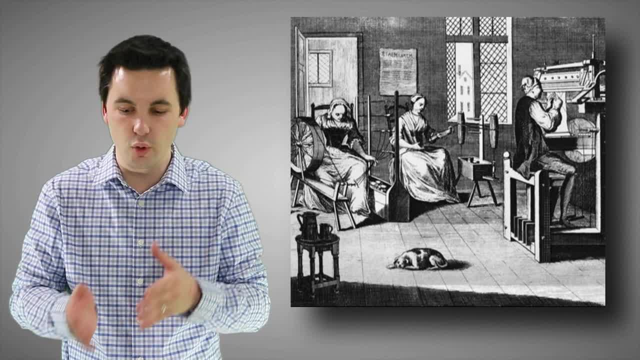 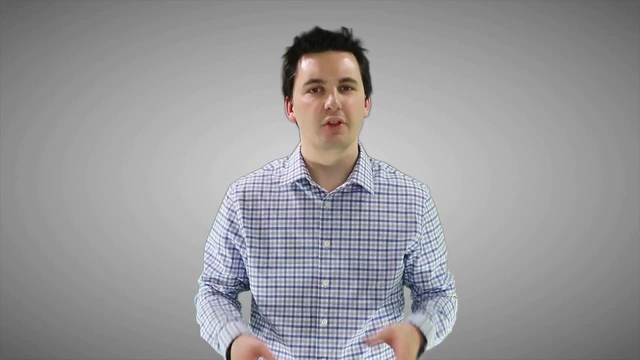 products. This motivated workers who had lost their jobs to move to urban areas and search for new opportunities in the city. In economics, we call this phenomenon creative destruction. This is when a new economy begins. Our economic pieces, sometimes greens and vans, are made of KI-Ki that can then be used as an arm. cottage industry make of involve&echdag 거야. 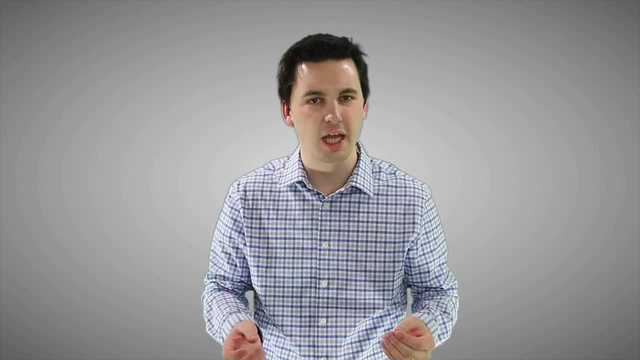 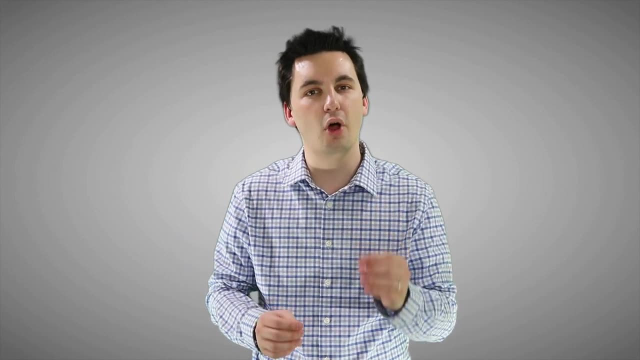 a new technology comes in and destroys an old industry. In the short run it can cause pain as we'll see people lose their jobs. Their skills are no longer needed in society. But in the long run we can see new opportunities created for society as a whole and oftentimes more economic. 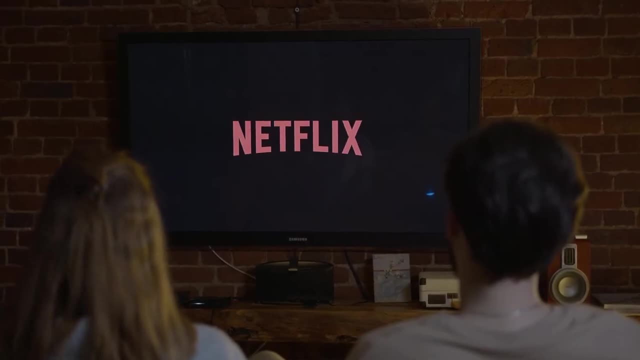 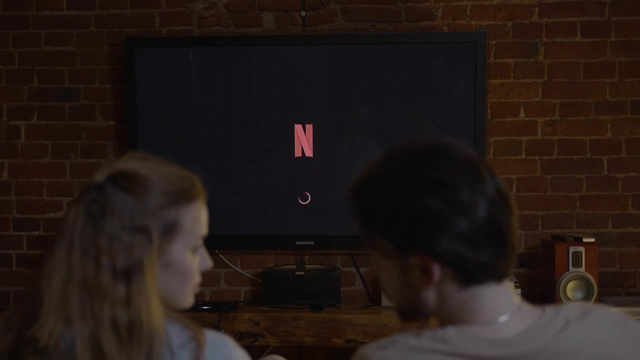 development will occur. Today we could see examples of creative destruction with companies like Netflix that completely changed how we rent and consume digital entertainment. Gone are the days of going into blockbusters or Mr Movies to rent a film. Some people even speculate we might. 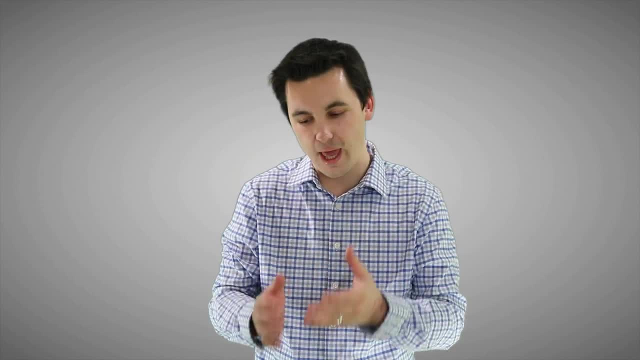 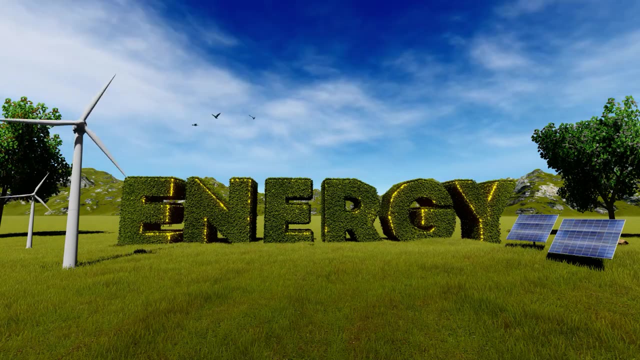 be seeing creative destruction happen again in the space of coal with energy. As more and more countries start to switch to green energy, coal power plants may become obsolete, Or we might be seeing this with the trucking industry. If self-driving, autonomous cars and semi-trucks 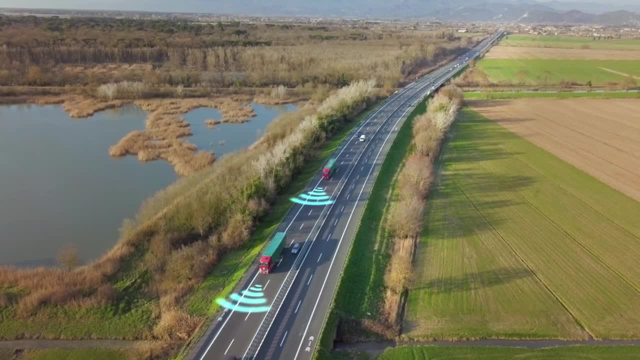 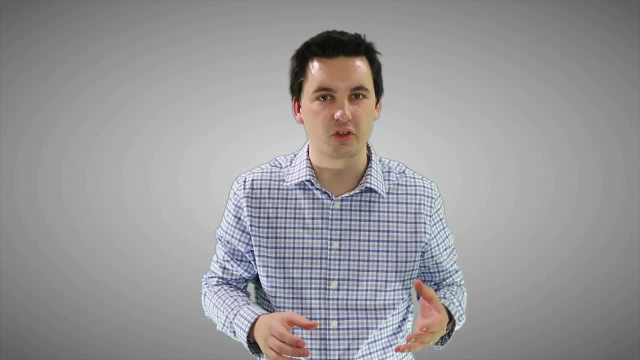 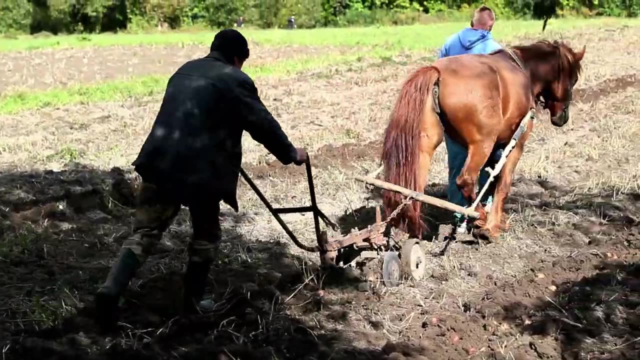 more goods. This led to the creation of more goods and services as we started to see the economy reshape itself. If we turn our focus over to agriculture, we can see how the industrial revolution transformed the field of agriculture. It led to the second agricultural revolution and 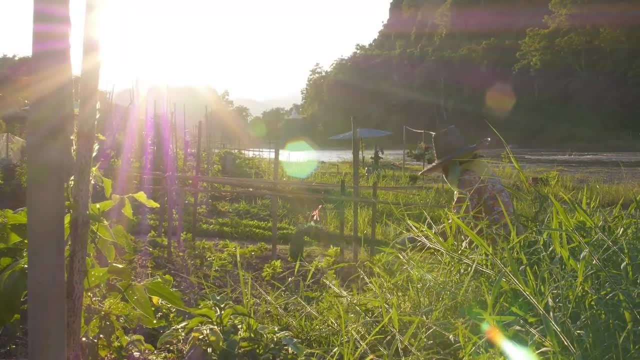 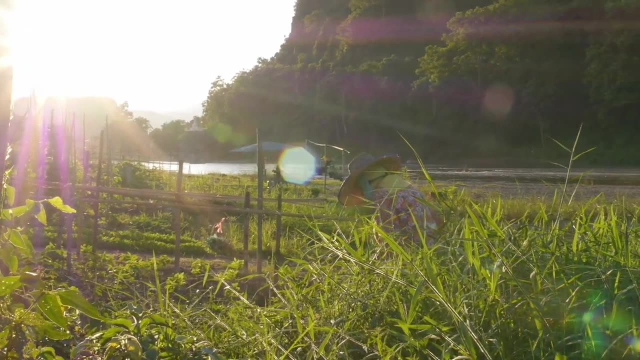 also the enclosure movement. This transformed how we produced food. We saw the introduction of new farming practices. We saw new technologies used to increase crop yields. We saw more food production and also a greater food surplus, which allowed us to have more specialization and also changed. 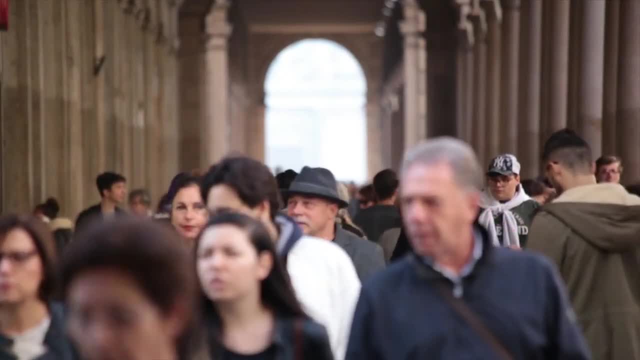 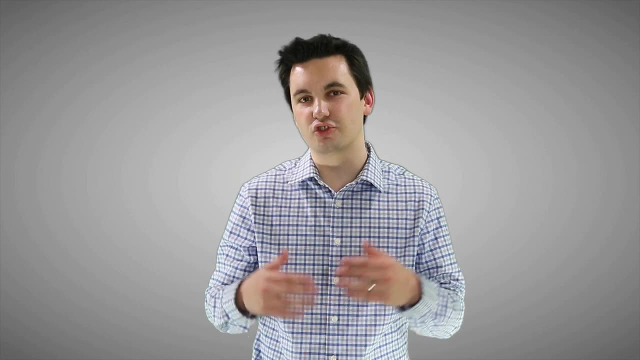 our migration again, as we saw more people move into urban areas as there was less farmers needed due to the benefits of the increased food production. We can also see that the industrial revolution's changes to society required a lot of raw resources. We can see that European countries 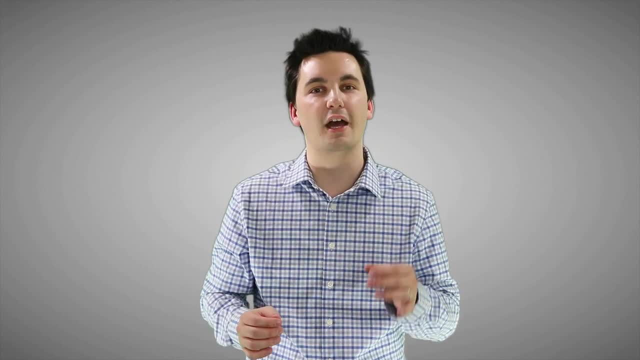 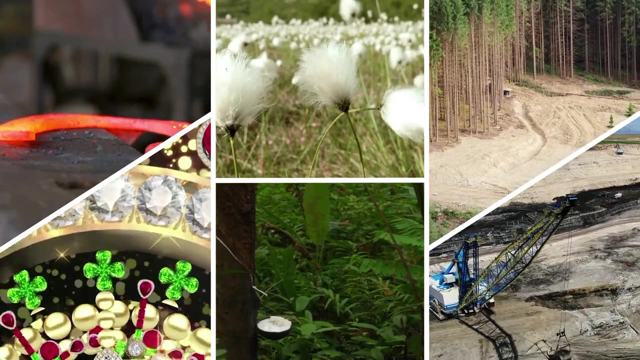 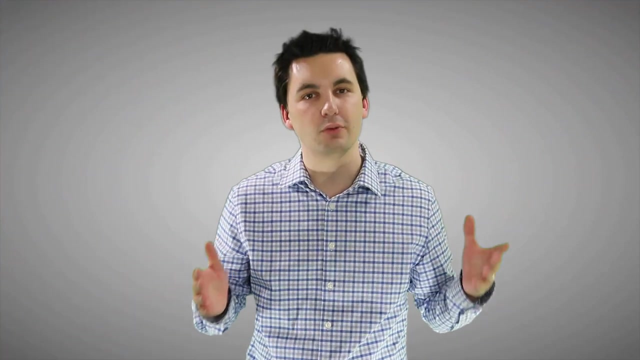 used colonialism and their colonies in order to make sure they had enough raw resources and markets to also sell some of these new products. Resources such as iron, cotton, rubber, diamonds, tea and wood became in high demand And with advancements in the steam engine we could see countries now could trade around the world and had access to. 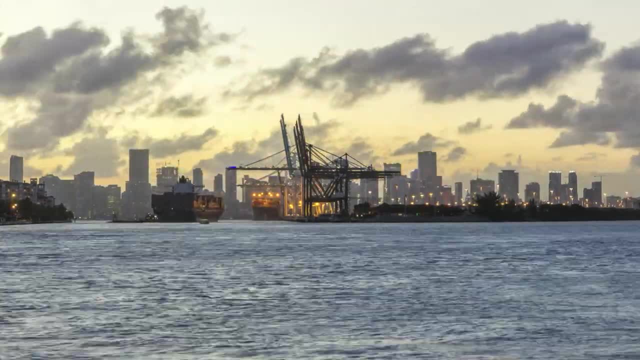 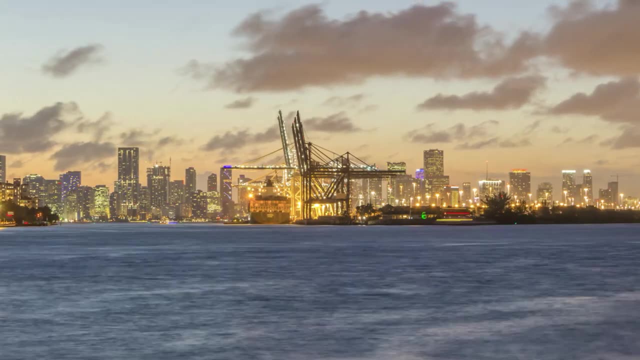 more markets than ever before. This led to the further development of ports being built in colonies, new technology being used to create canals, railroads and infrastructure, all to support global trade. Remember back to our political unit, when we were talking about 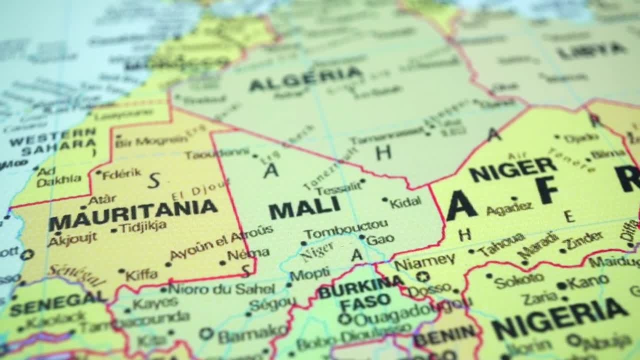 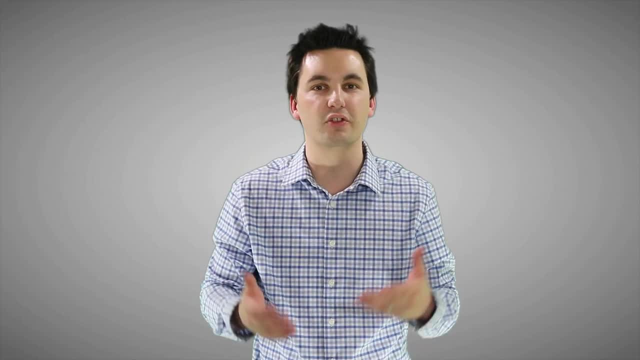 colonialism and imperialism and the scramble for Africa, where we saw Europe's economic growth grow. We saw European powers use their influence over Africa to benefit their own economies. They needed those raw resources in order to continue their economic growth. If you need a refresher on some of those concepts, go back and check out some of the Unit 4 videos. 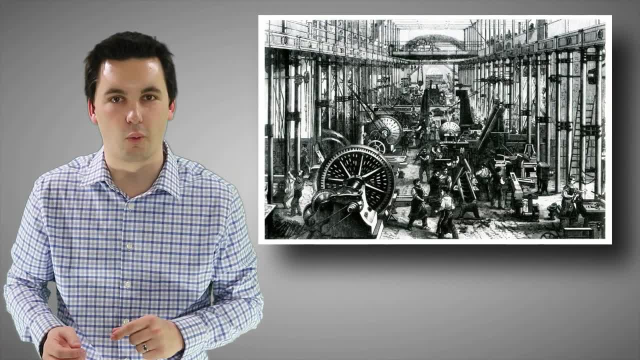 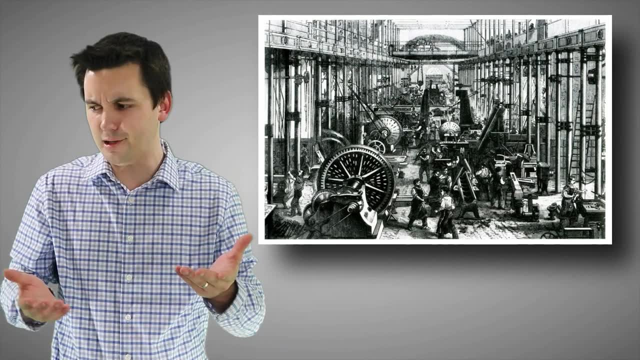 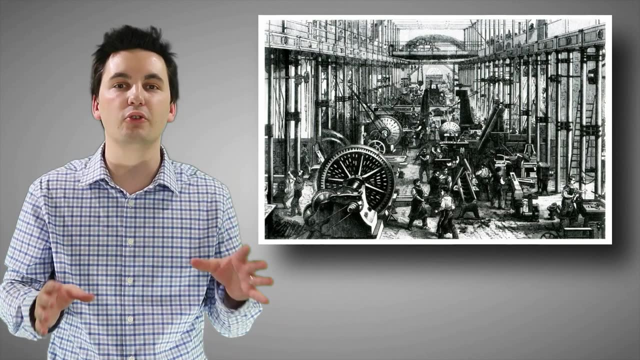 As you can see, the industrial revolution truly did revolutionize the world. We can see concepts from this topic in Unit 7 connect to almost every single unit in our class. It's kind of like the greatest hits of our topics. We've talked about agriculture, culture. we've looked at population migration. we've also talked about the importance of economic growth. 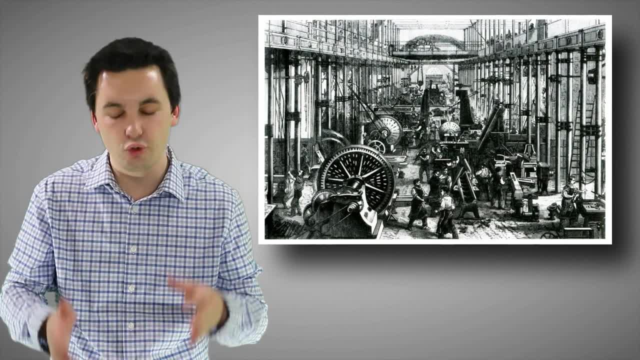 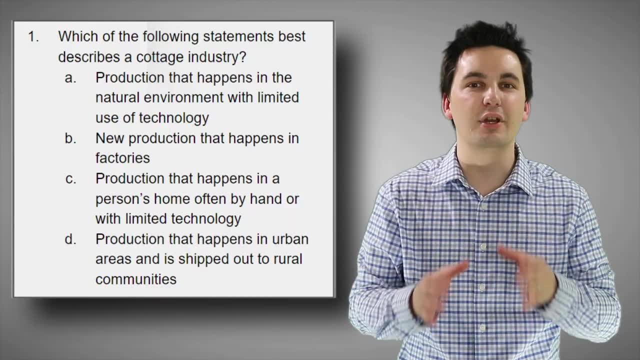 We've also talked about our political unit in here. The industrial revolution was major, and it changed our society forever, And now comes the time, though, that we need to practice. Take a couple of minutes now and answer the questions on the screen right now. When you think you got the answers, go down into the comments. 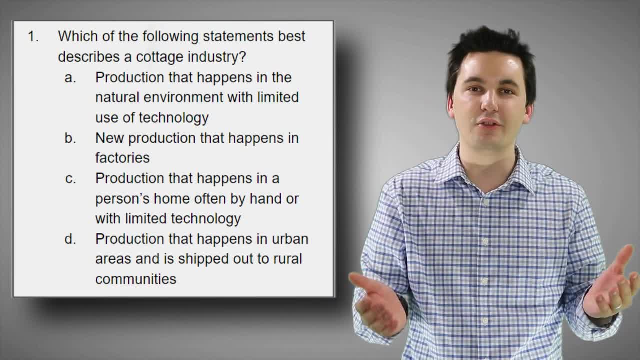 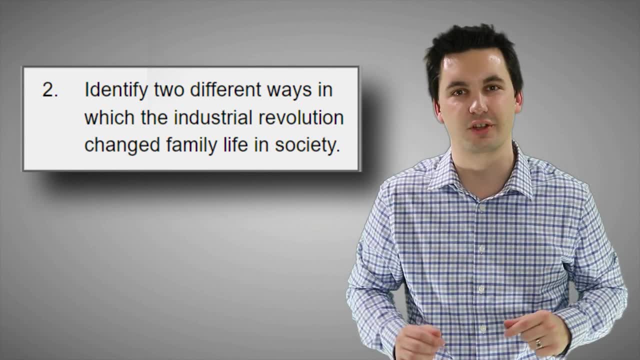 section and check your answers, Make sure you got them right. And when you're down there checking your answers, don't forget to hit that subscribe button and also check out my ultimate review packet. You can find a link for it in the description of this video. It is a great. 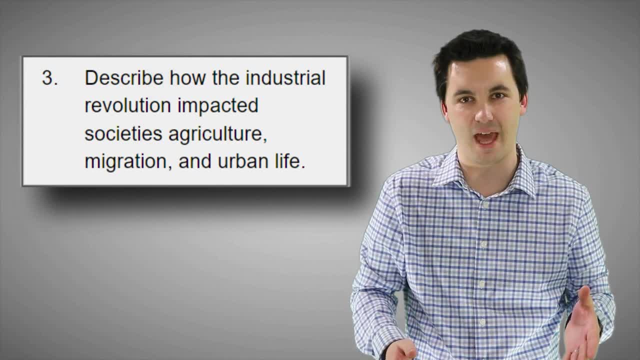 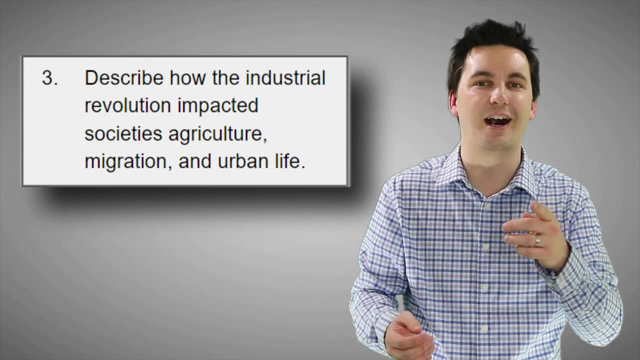 resource that will help you in your class and also help you on that national exam. All right, geographers. that's all the time we have for today. I'm Mr Sin. Thank you so much for watching this And until next time I'll see you guys online.